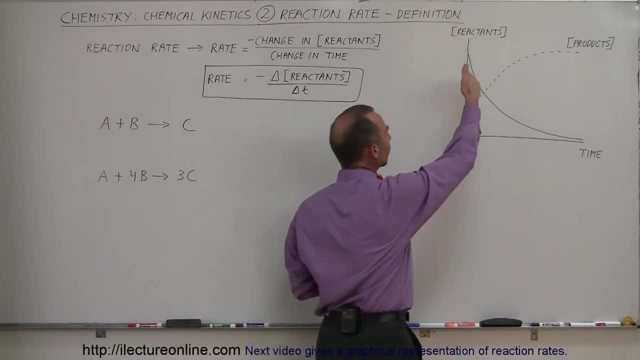 the slope is negative. When the line goes this way, the slope is positive. So you can see that if we look at the concentration of the reactants over time, the slope of that line is indeed negative. And since we can't talk about the negative reaction rate, we have to put a negative. 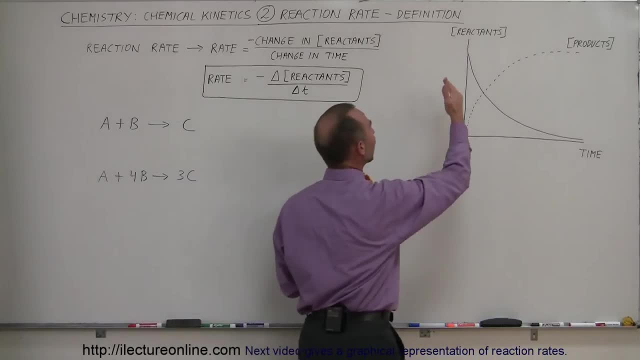 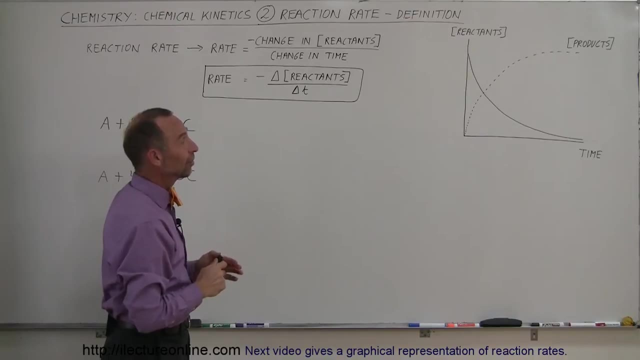 sign in front of it to make it make sense. So we simply make it the negative of that slope divided by the change in the time. Or actually the negative slope is the change in the reactants divided by the change in time. So let's say we have a reaction where we have two reactants and 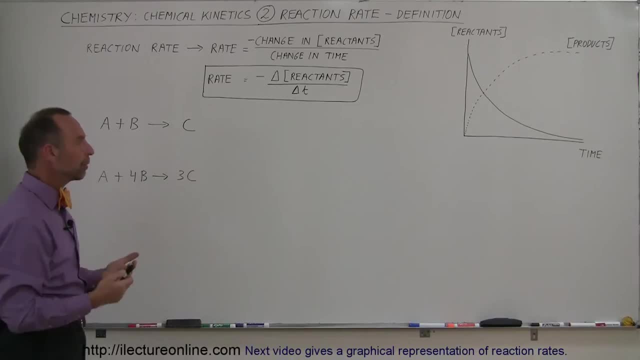 one product, A plus B, form C, How do we express the rate of that reaction? Notice that we don't say reaction rate, we simply say rate, indicating that's the rate of the reaction. So we can look at the reactants, we can look at the products. You can see that you need one of these and one of 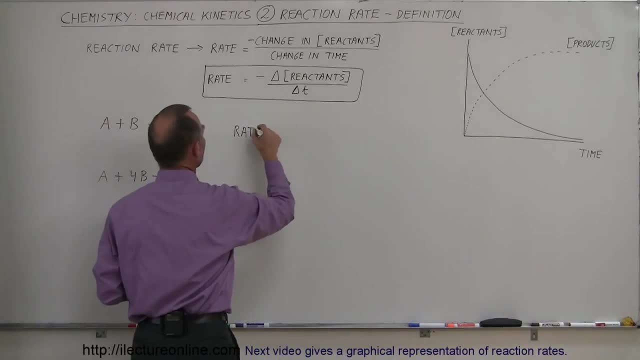 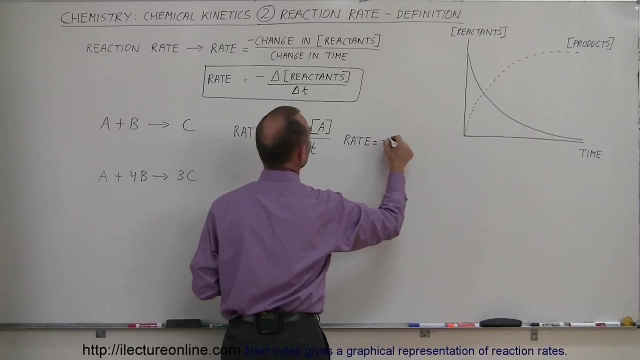 these to make one of those. So in that case you can express the rate as being equal to negative the change in the concentration of one of the reactants, let's say A divided by the change in time. Or you can say that the rate is equal to the negative change in the concentration of the. 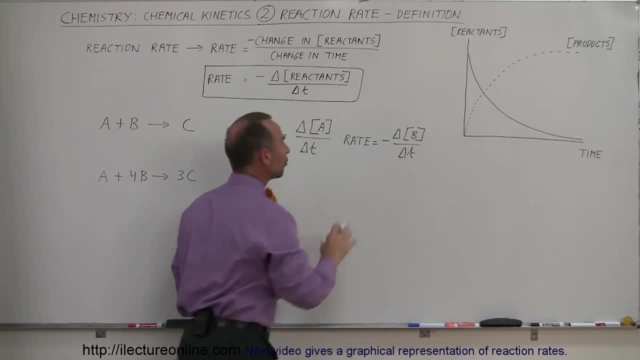 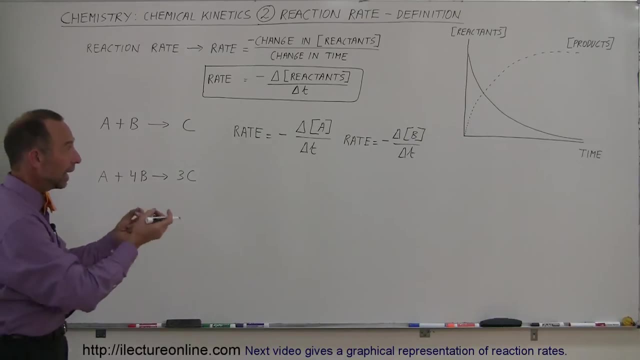 other reactant divided by the change in time. Notice, since you need the same amount of reactants for A and for B, or from A and from B, then the rate can be expressed in either one and it'll be the same. like that, You can also express the rate in terms of the products being. 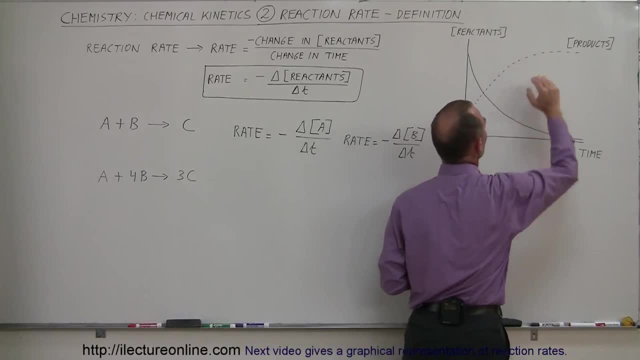 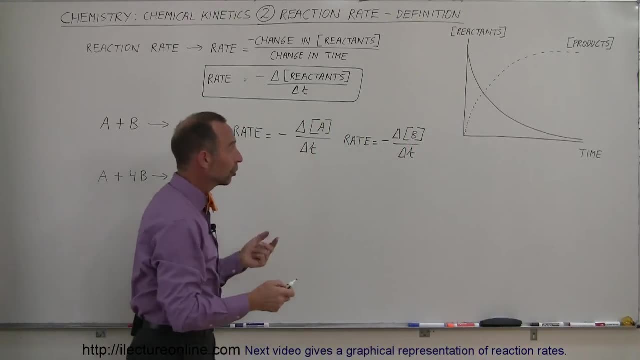 produced Here. you see this dashed line here representing the concentration of the products. Notice that the positive slope here is equal to the negative slope there. so simply difference by a sign, And so you can also say that the rate of that reaction can be expressed. 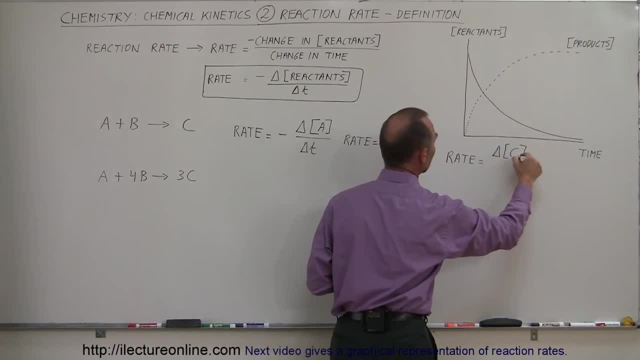 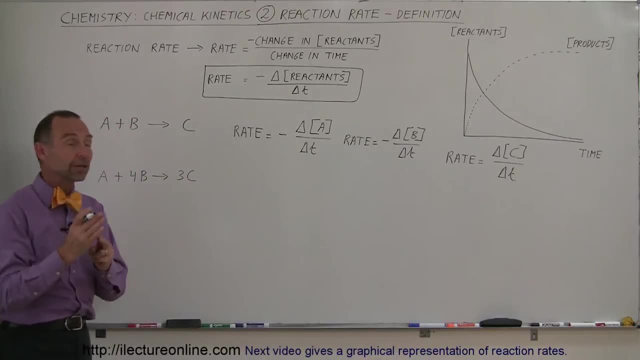 as the positive change in the product, in this case C divided by the change in time. So here we don't need a negative sign because we already know that the slope is positive. it's just that numerically the slope is the same, it just differs by a sign. 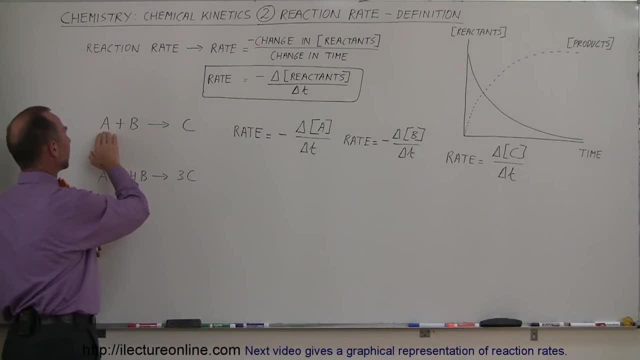 So we don't need just one of A and one of B to make one of C. For example, one atom of A plus one atom of B makes C. or one molecule of A plus one molecule of B makes one molecule of C. or in terms of moles, Sometimes we'll need more of one reactant than another. So how do we express? 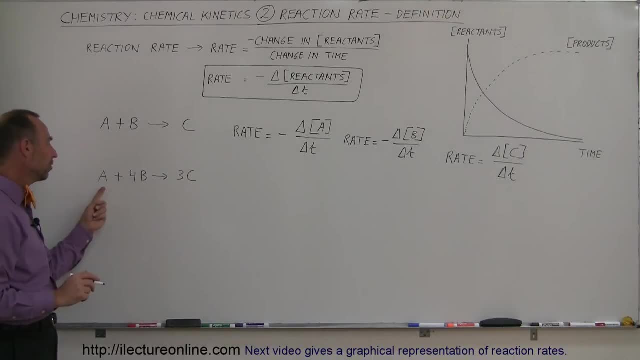 the rate there. Well, if you need four times as much of this reactant compared to this reactant, this reactant will be consumed four times as fast, And so, therefore, the rate needs to be expressed in terms of the concentration of this or the concentration of that. 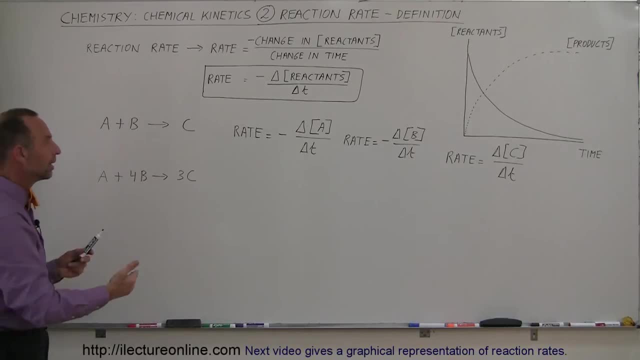 So if we need four times as many of these for the same rate of the reaction, then the rate will be expressed in terms of four times the concentration of this versus one time the concentration of this. I'll show you what that means. So we can say that the rate of the second reaction can be expressed. 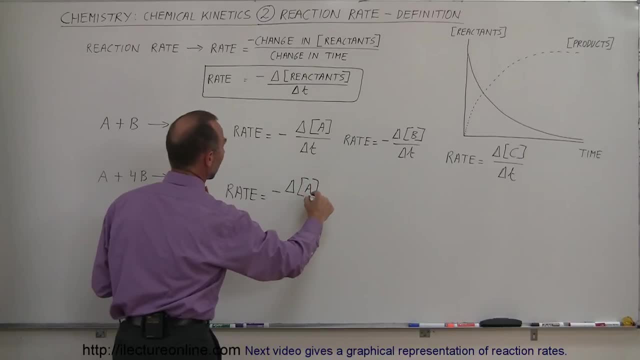 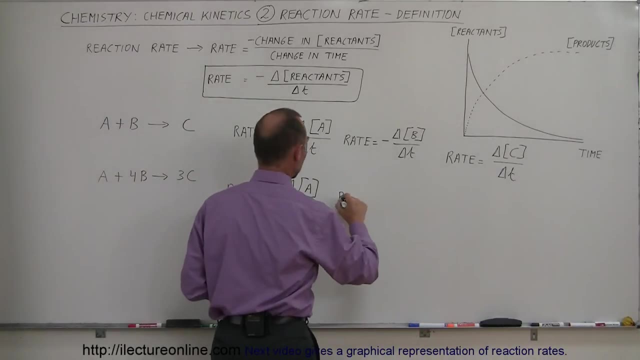 in terms of minus the change in the concentration of A with respect to time, or with respect to the change in time, I should say. And then here, in the case of B, we want to look at that reactant. There we go. 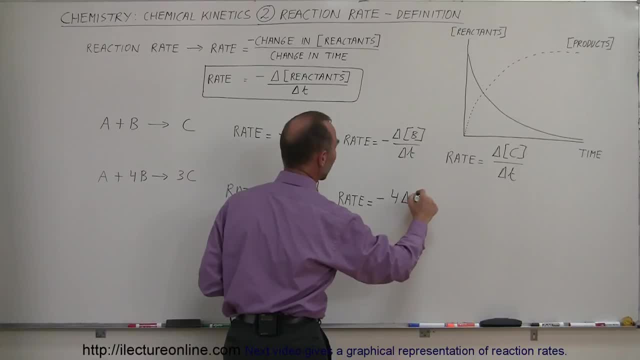 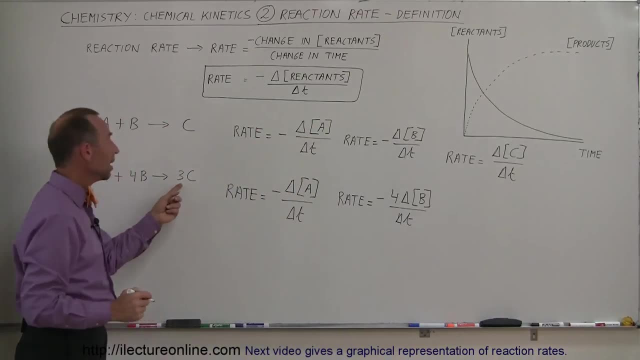 The rate is equal to minus four times the change in the concentration of B divided by the change in time. And then if you can see that there's three of the products being produced for every one reaction, then you can also indicate that the rate of that reaction. 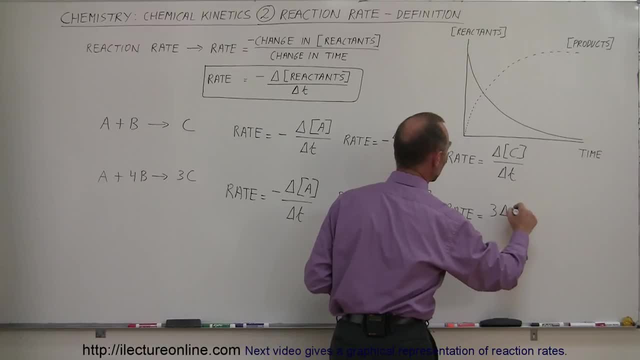 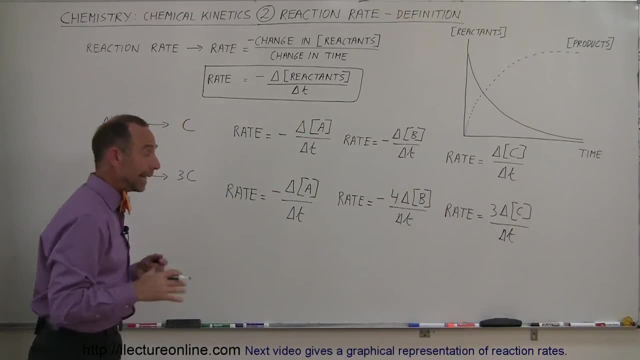 can be expressed as a positive three times the change in the concentration of C divided by the change in the time. So you can see. that's how we mathematically indicate the reaction rate, either using the products or using the reactants. And, of course, if you have a situation where there's 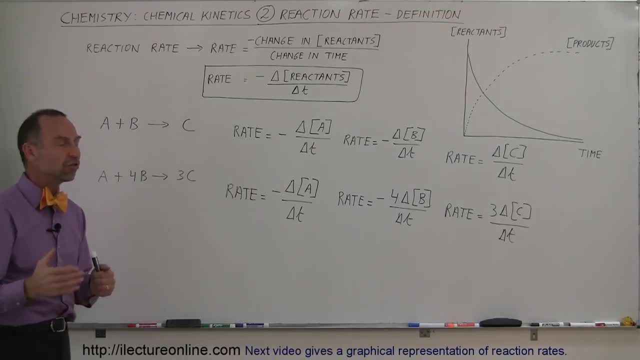 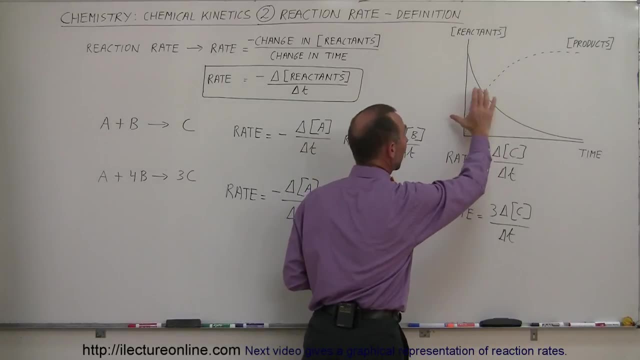 more of one reactant that you need compared to the other. you can see how you then change the way you represent the reaction rate. So now in the next video, we're actually going to take a closer look at the slope and how we can actually indicate graphically what the reaction rate is. 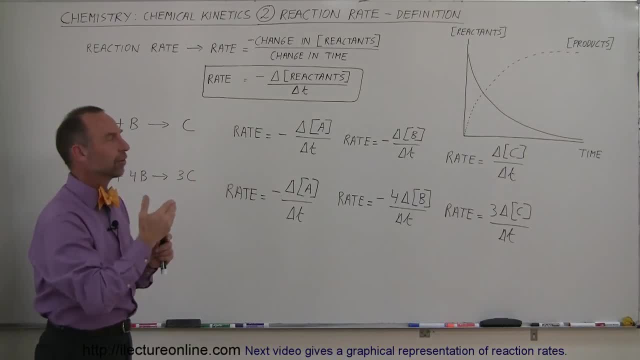 by looking at that slope, by taking maybe intervals over intervals of time, the amount of reactants that you have or the amount of products that you have, to figure out how to come up with a way to express the reaction rate So graphically. that's our next video.